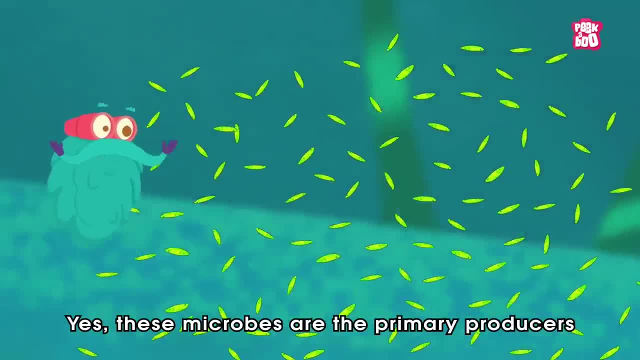 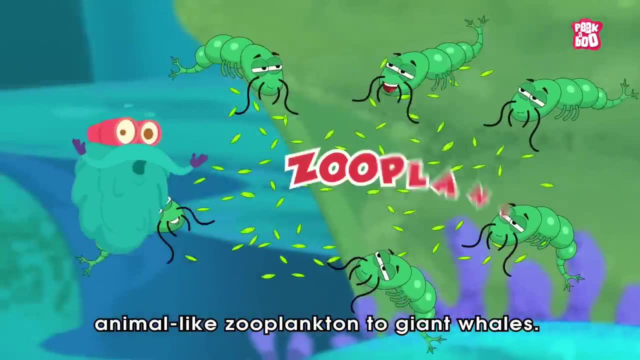 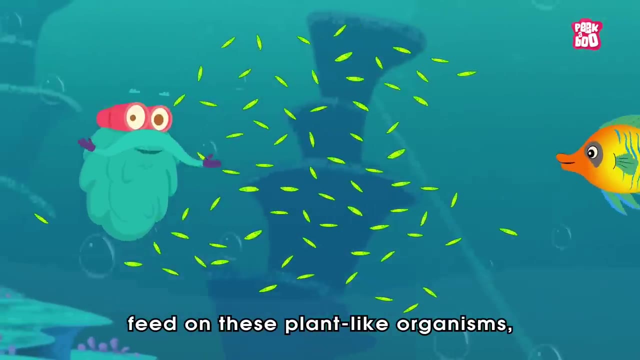 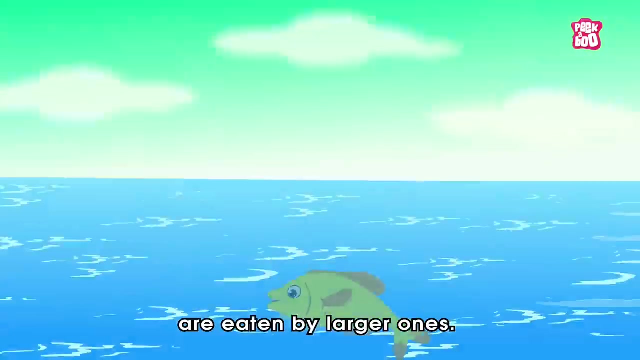 Yes, these microbes are the primary producers and serve as food for everything from tiny animal-like zooplankton to giant whales. Even small fish and invertebrates also feed on these plant-like organisms And in turn, these smaller aquatic animals are eaten by larger ones. 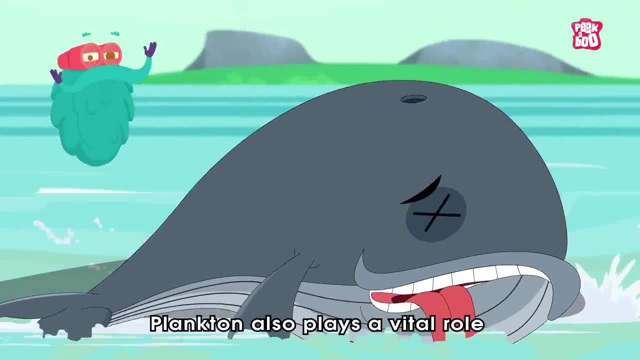 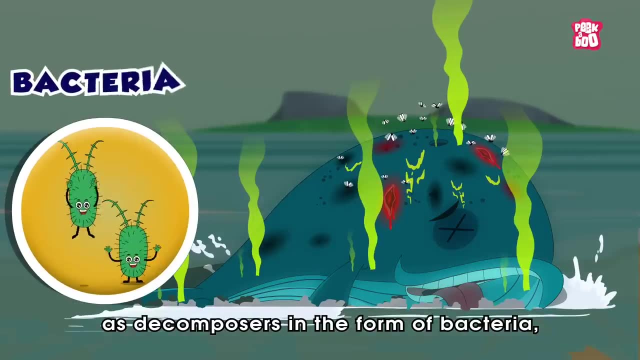 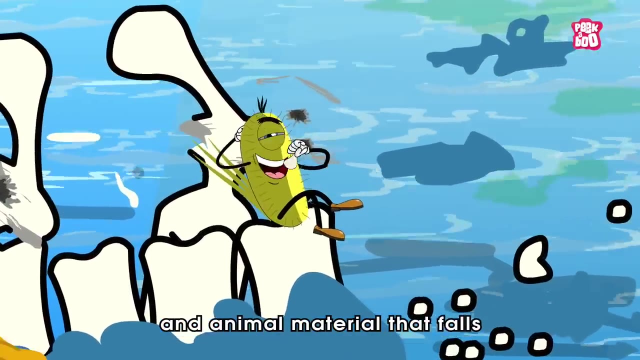 Not only that, Plankton also plays a vital role at the end of the food web as decomposers in the form of bacteria, fungi and worms That break down and consume dead plant and animal material that falls through the water column as marine snow. 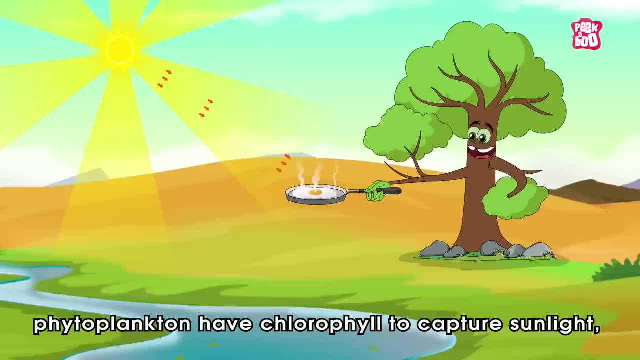 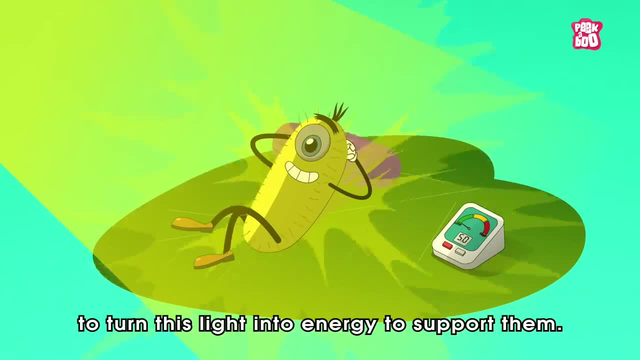 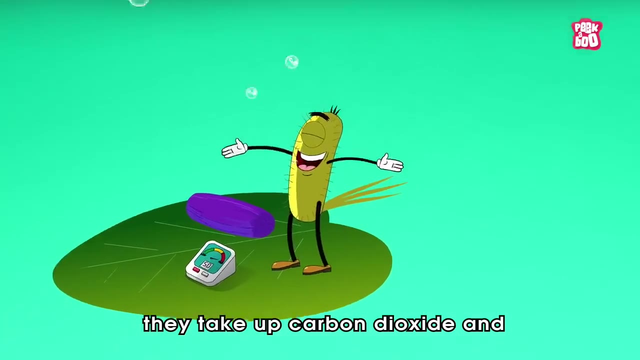 On top of that, just like terrestrial plants, phytoplankton have chlorophyll to capture sunlight And they use photosynthesis to turn this light into energy to support them, And in this process they take up carbon dioxide and release life-supporting oxygen into the water as a waste by-product. 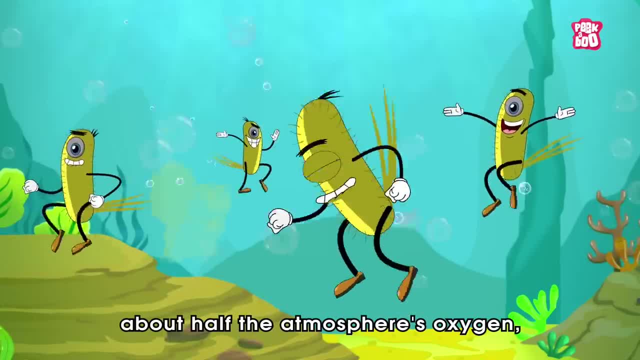 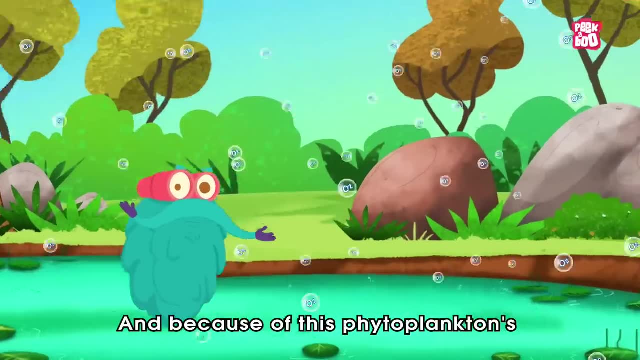 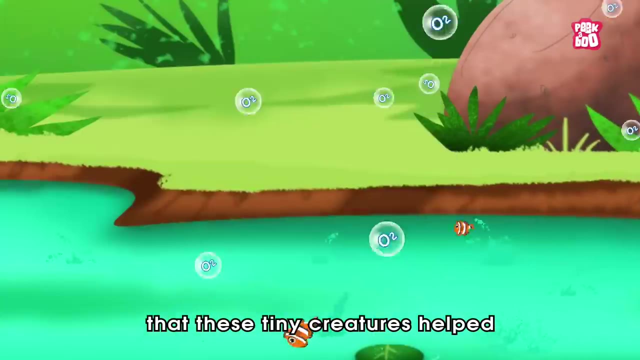 And you won't believe it. They generate about half the atmosphere's oxygen- as much per year as all terrestrial plants- And because of this phytoplankton's enriching quality, many scientists believe that these tiny creatures helped in the formation of complex life on earth. 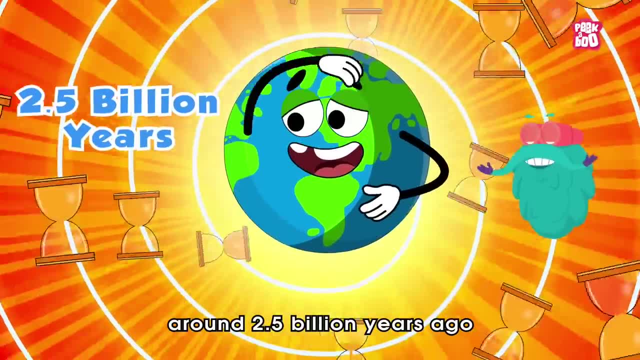 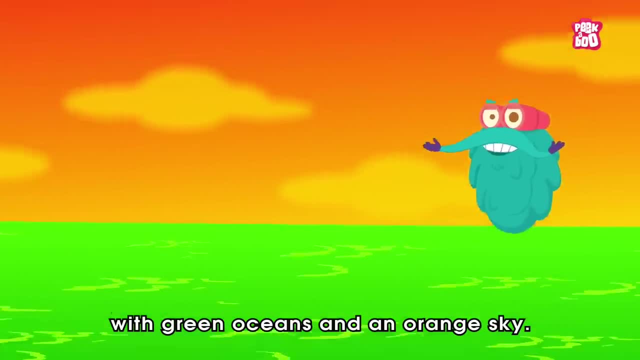 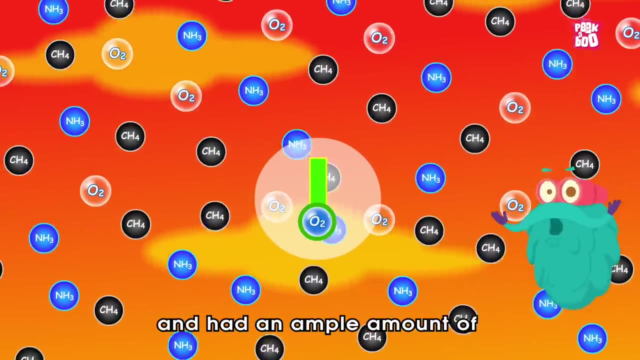 Yes, that is because around 2.5 billion years ago, the earth looked way different than today, With green oceans and an orange sky, And even the atmosphere lacked enough level of oxygen and had an ample amount of methane and ammonia, Which is not suitable for complex living beings like us. 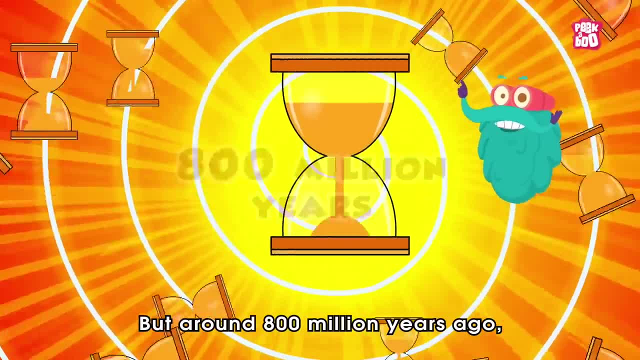 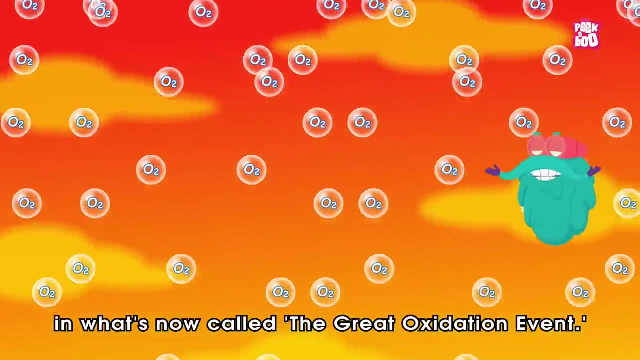 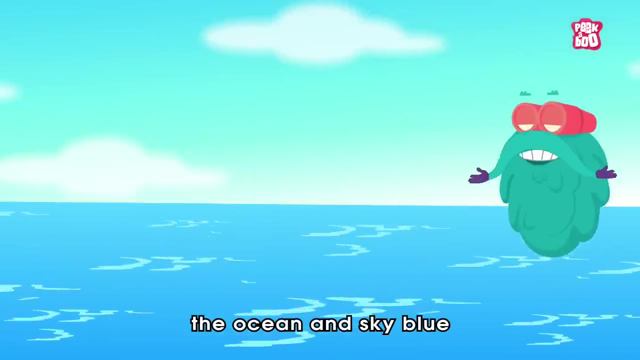 But around 800 million years ago, some phytoplanktons evolved and pumped out enough oxygen in what's now called the great oxidation event. All this oxygen eventually turned the ocean and sky blue and allowed the complex life to develop in water and subsequently on land.